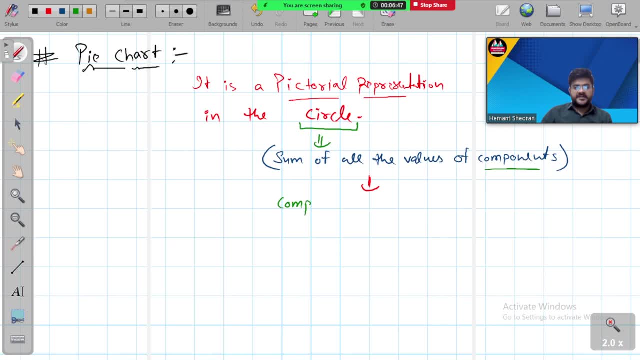 These components. So the components are represented where Sectors, Yeah, Are represented in form of, In form of sectors, Sectors, Sectors, Sectors. Okay, Now the next question is: what do we mean by a sector? What do you will say? 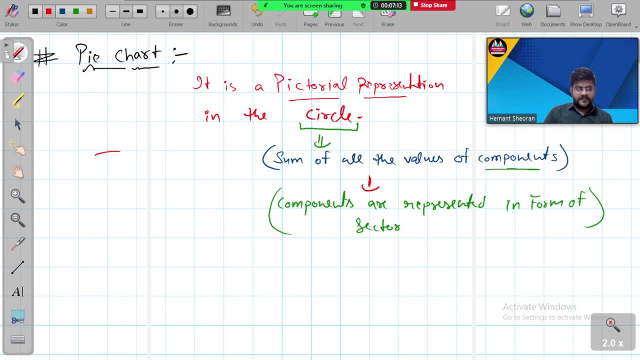 Part of the circle, like, Like. if I made this circle Line of the radius to the Parts, You can say a part between the boundary and the two radii, Yes or no. So this specific like boundary And these two radius are covering, like, are making a particular part out of it. 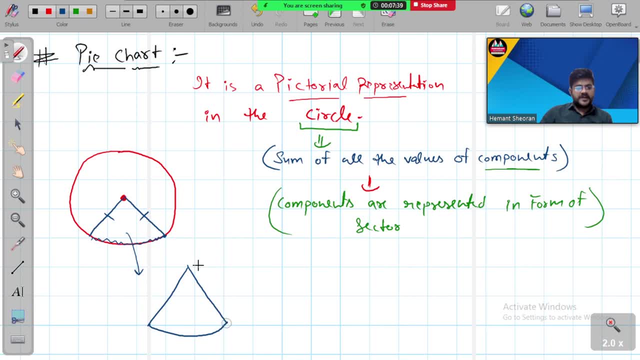 Yes or no, And this part of a circle is known as what it is known as a sector for us, Yes or no, And the two radius will make a specific angle over there, Yes or no? Yeah, And we call it what we call: that angle. 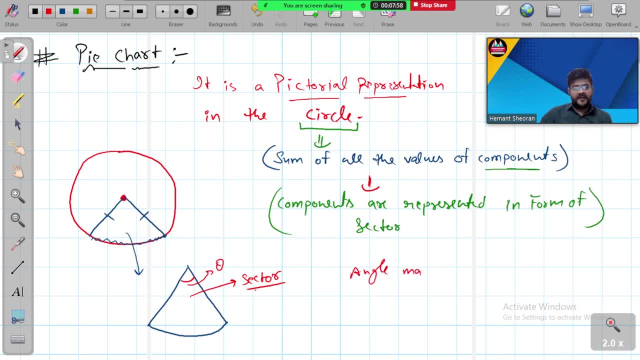 So the angle Made by The radius And what in that Sector is what Is known as a central angle. Okay, What we call it? We call it as a central angle. Any confusion? No, So just the important parts are: what is a sector where we represent those components? 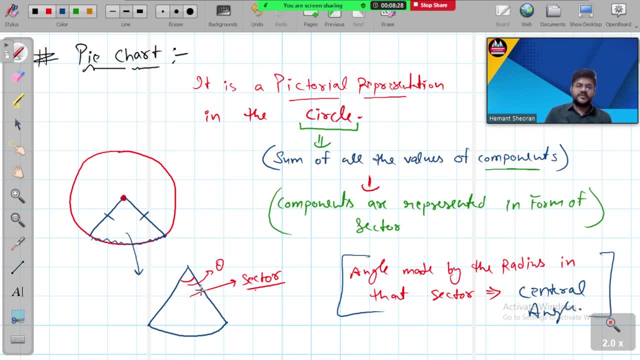 So components are represented in the form of sector. Sector is what The part made between the two radius and the- You can say- boundary of circle. We call it as a sector. Get it. There are basically two sectors that you are framing now. 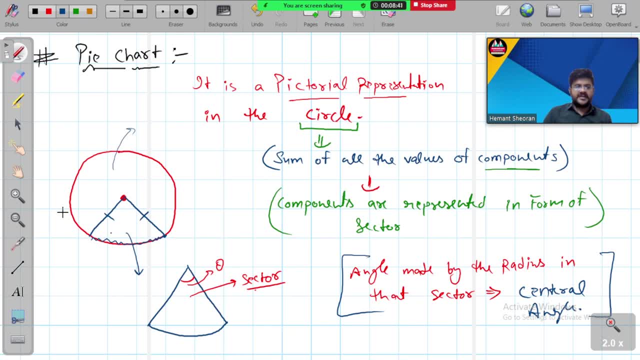 Like if you cut it out, So one is a bigger sector, One is a smaller sector. The bigger one is known as a major sector, The smaller one is known as a minor sector, But that you will specifically read about in, You can say the circle. 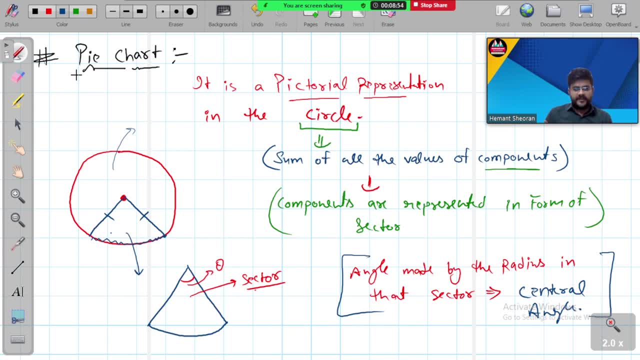 Okay, Now we are just reading pie chart, So we don't need to go in deep in that. Okay, Yeah. So now the question arises: How do we calculate this central angle with the help of the data that we are representing, Representing over there? 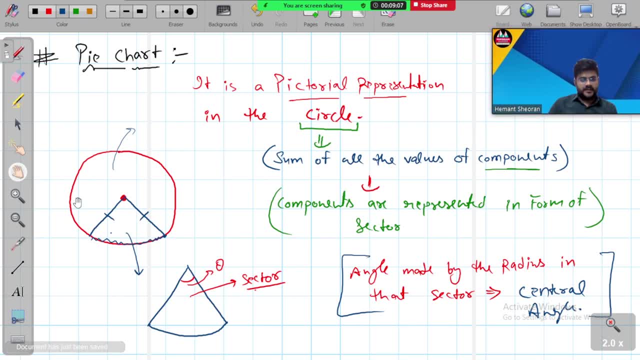 We do the Yeah. Imagine there's like different amounts and there's pineapple pizza. Let's say how much pineapple pizza over the total amount of all the pizzas times 360, because there's 360 degrees in a sector. Okay, So basically like in general, what we can say. 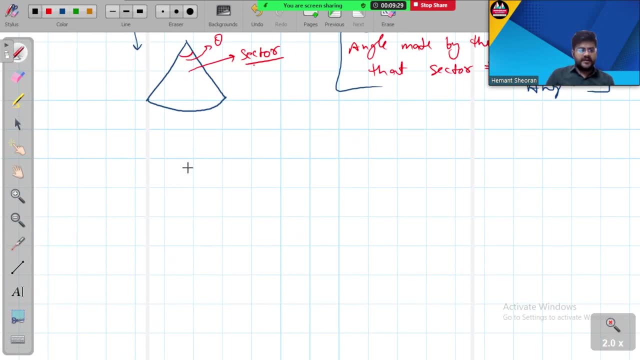 The simple formula. in general, We can write it as: the central angle will be equal to what you can say. It will be equal to the central angle for a component. You can say, but for a part, will be equal to what will be equal to the, the value of component that you want to represent, divided by what, divided by some of all the values. 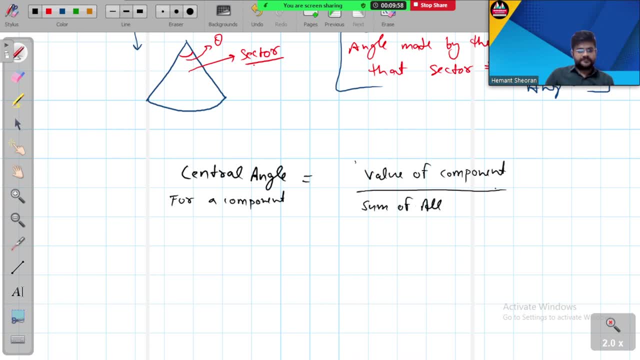 Okay, And as it is a part of a circle, So we need to know what angle we have at the whole circle have. so we know it is 360.. So we times it by what? times it by 360 degree, Yes or No? 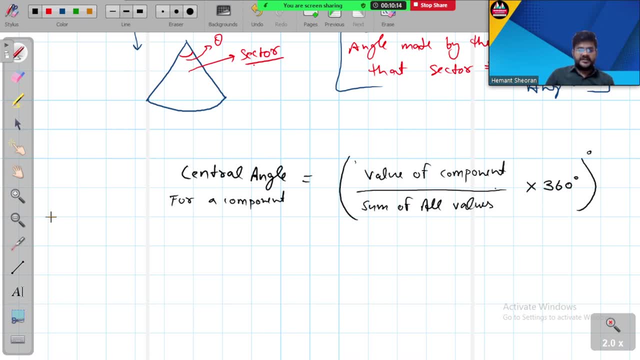 So it is a part of that 360 degree angle. So this is the general formula that you can remember: do 360 divided by sum of all values and then the sum of the worship value of all of the values. So this is an example. 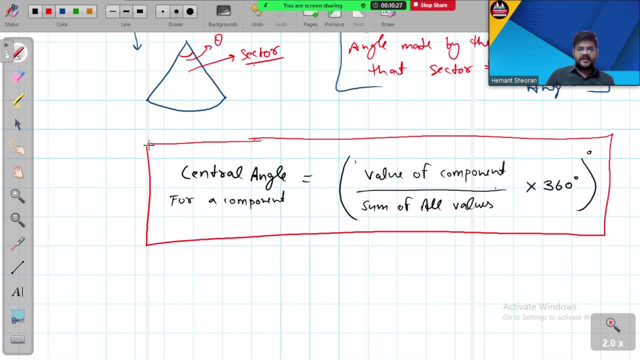 Okay, times it by the value of components. that is the same. like you're just replacing the numerator over here, you're putting this 360 as a numerator and the other value as a product. yes or no? yeah, yep, good, okay, then do you know what are the steps to construct it? 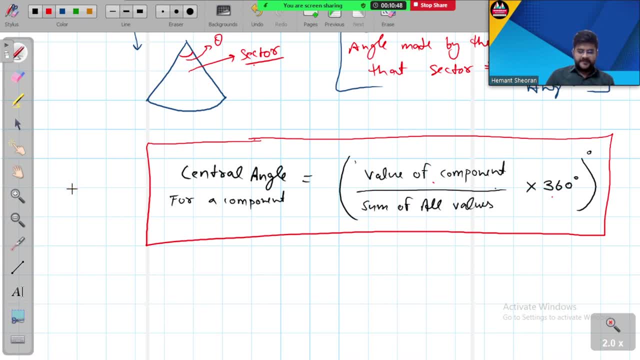 um, we first use a compass and then draw a circle. draw a circle of a convenient radius, that much you want. okay, there is no restriction on the radius that you want, get it. and then we use a protractor. and before that, before, before the, before the- uh, just listen it. before the protector. 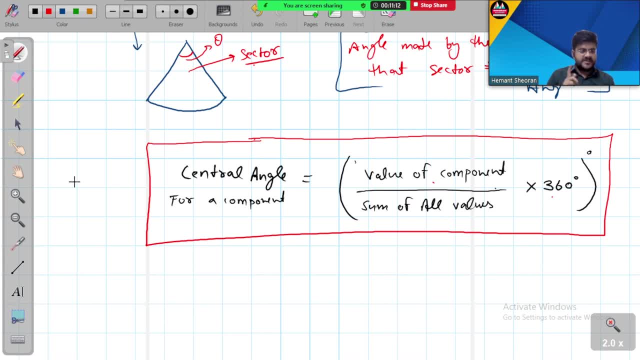 what we have to do. we need to make a radius. okay, just create a single radius by the ruler. or you can say like this: and then we can make a radius, okay, and then we can make a radius okay, and then say, okay, so within the circle, draw a horizontal radius and then try creating those central angles. 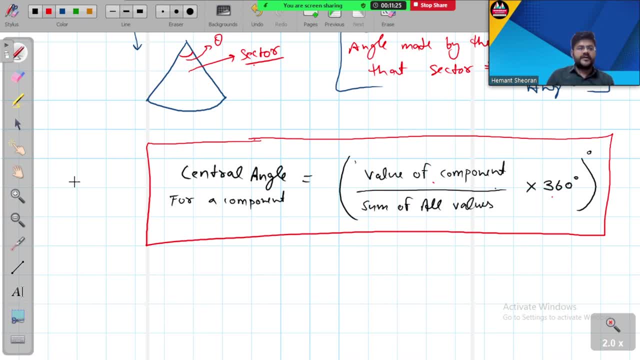 that we have already calculated. okay, for each component you have to calculate the central angle and then, with the help of that radius, you will start drawing them. okay, get it. so just make a horizontal radius and, with the help of that horizontal radius, just create one angle. then 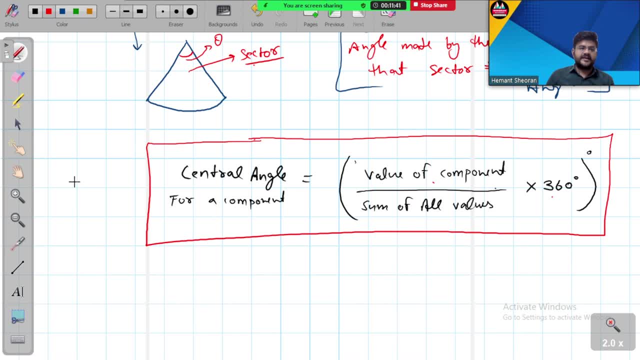 take the other one as a radius and then create the other angle that is just adjacent to it. got it okay, yes or no? and these radius that you will create, now, the new radii that you will create, will frame what will frame the whole pie chart for you. get it? yeah, okay, we will understand it. 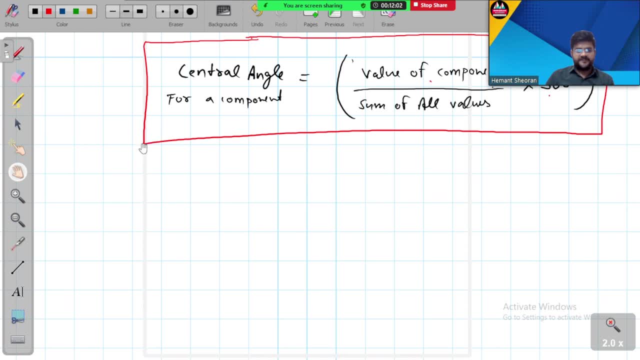 better, better with the example. you can say so: let's no, i get it, you get it. okay, let's do an example as well, because let's do a question as well on it. yeah, okay. so if i give you a simple question, let's say like, uh, you have to create it as well. or like you just have to do the. 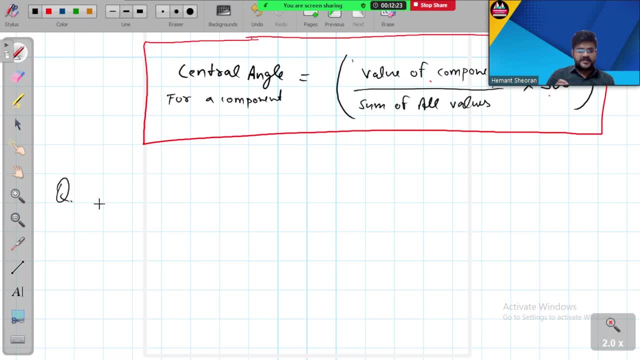 observation only: which part is coming for you both? okay, both are coming for you. okay, good, so if we start with it. so they are saying a men, uh, we have some men with the after, take out my equipment. no, we are just doing it roughly. okay, then later on, like you can practice, just for one. 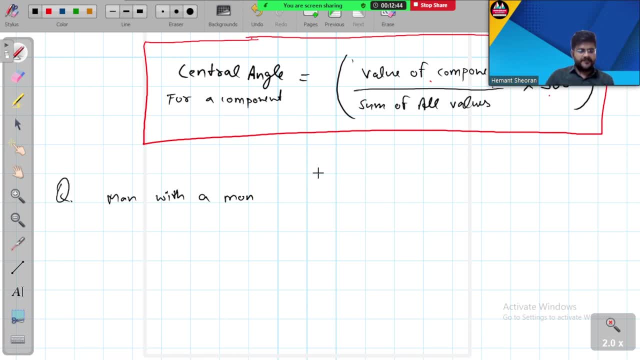 of them you can take out. so just take it out for this one, okay. so mn is there with you can say the monthly salary of how much rupee let's take. uh, ten thousand eight hundred, okay, and he plans what. he plans his budget for a month. 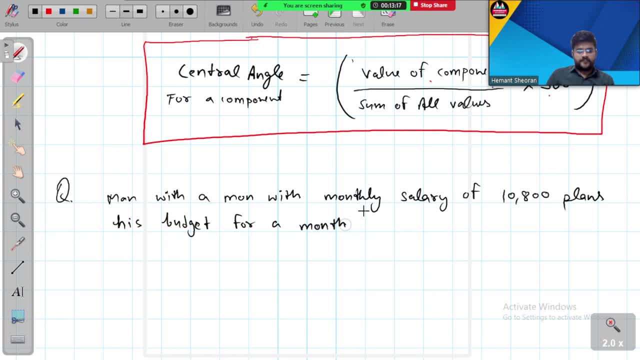 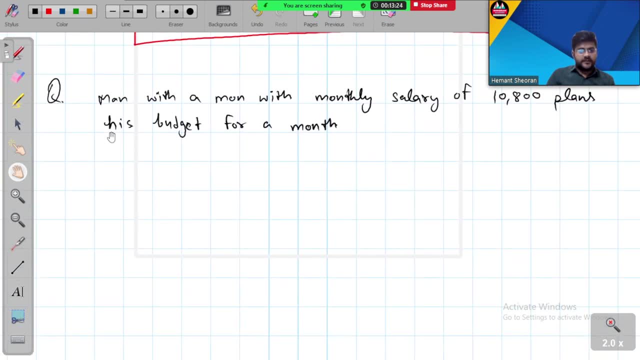 okay, so mn is there with you can say the monthly salary of how much rupee. let's take ten thousand, as given below. you can say, like now we will be working on the table that they have provided us. let me create the table first. so, first of all, the thing that he's going to purchase, we call it. 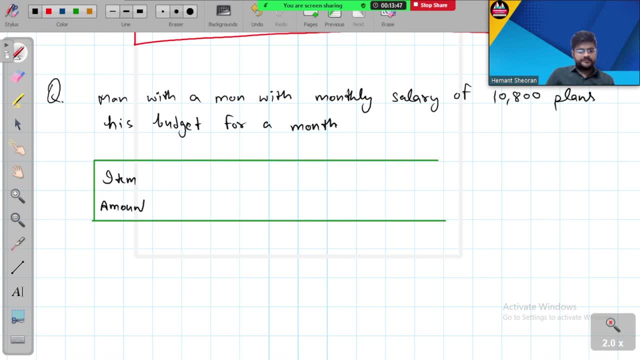 so first of all, the thing that he's going to purchase- we call it item- then how much it costs, that is the amount. okay, now if we write down the specific parts. so firstly, let's say, like he's spending it in food. then he spends like, let's say, 3150. 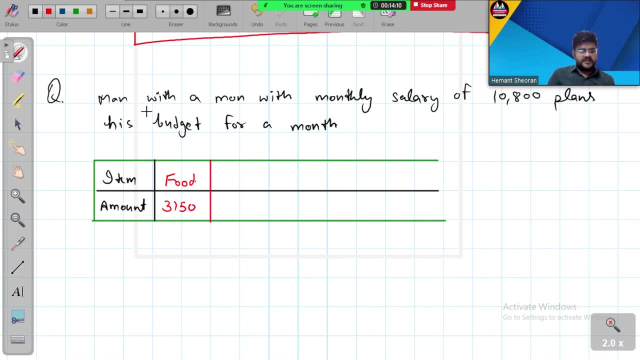 and then the next thing that he do is a rent that he pays. so for rent he's spending 2100. then the next is you can say the education. so on education he planned to expend 1950. okay. then the next one: he plans to do savings. so he do a saving. 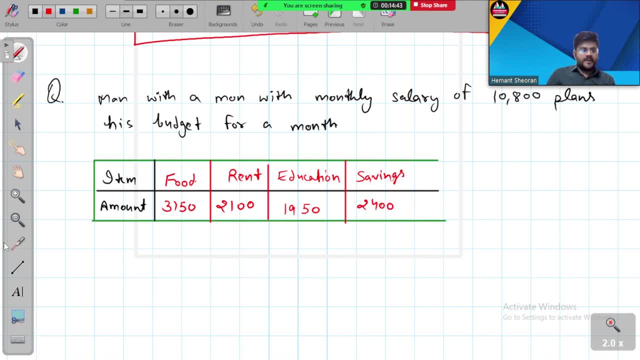 of what? 2400. and then there is one more expense that he do, that he do not care about, like miscellaneous, you can say, or he doesn't count over there, like at what part he's spending. so let's say 1200, he do for that. so now what you need to do: 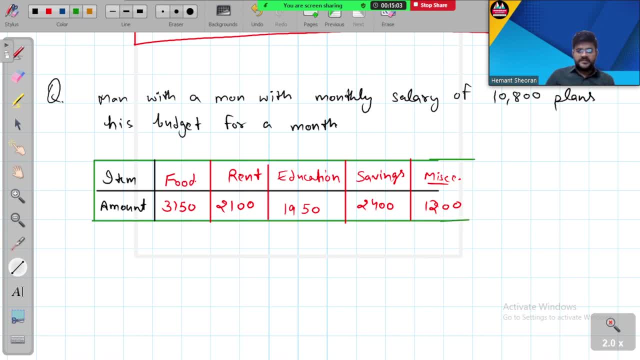 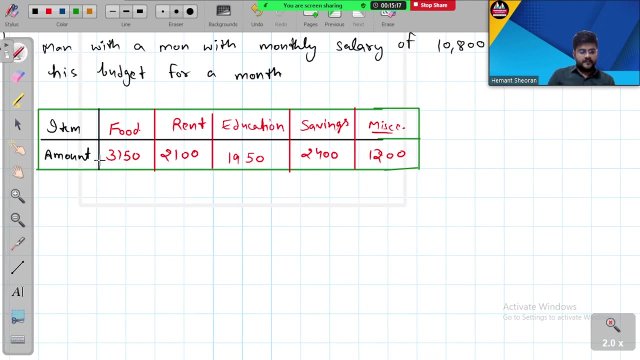 you need to prepare a pie chart for it or represent the above data. you can say in a pie chart so how we gonna do the representation for it. we for food, we can do three, one, five over ten, eighty. so firstly, like we can calculate the central angle, yes or no? yeah, okay, so let's do the calculation. 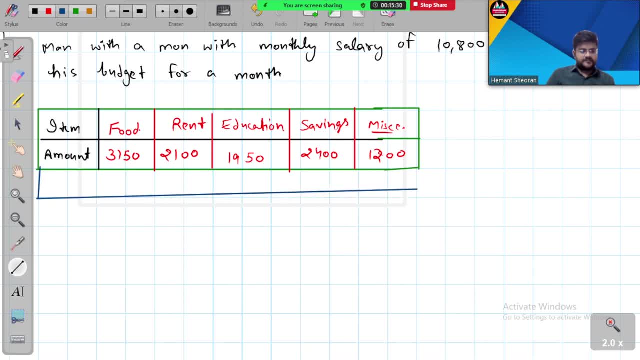 for the central angles for each part specifically. okay, so if I calculate the central angle, so central angle will be how much you can say. it would be like three, one, five, zero. is it required? let's see. if it will be required, then we will use it, otherwise we can skip it. okay, so there are two zeros I can cut. 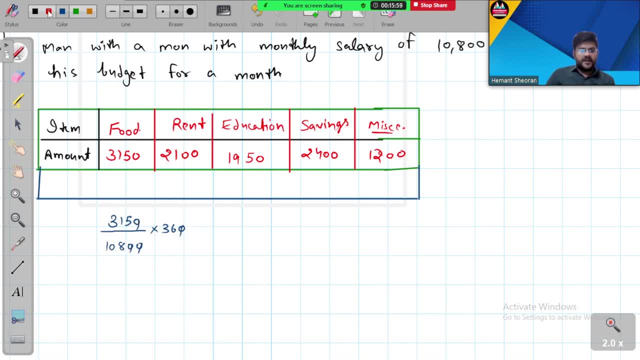 out the two zeros, get it now. if you know the 12 stable, 12 times 3 is 36, 12 times 9 is 108, yes or no? then if you know the three stable so you can cut it out at 3, get it. 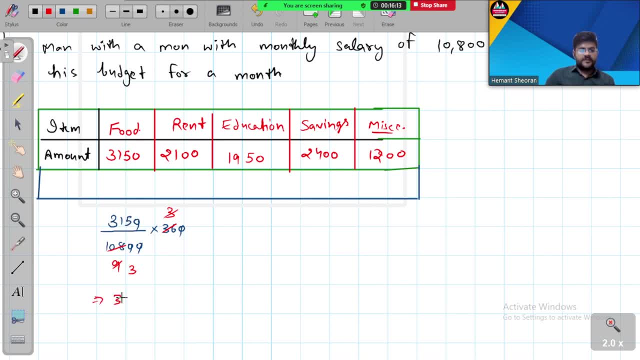 so now we are just left with what three one, five over a three, get it yes or no? so what answer you will have? and we got it out: three ones are three, then zero and then five. so 105. I got yes or no, so I will fill it with a 105 now in the 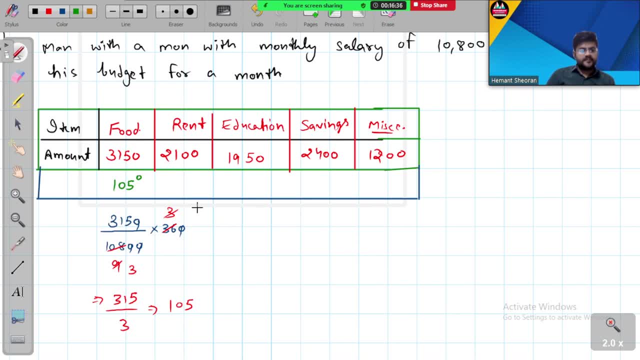 same sense we can calculate for others as well. for the next one, it would be what? 2100 over 10800 times by 360. if you cut out the thing so 36, again cut out the 108 at 3, then 3 will cut out the 210 at 70, so you got a 70 degree. can i finish the table? yeah, yeah, just be. 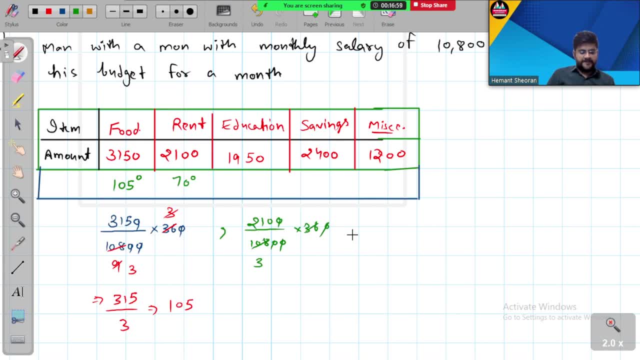 quick, we are just dividing them by 3 now, like they all have 0. so just remove one of the 0 and 36 will cut out 108 at 9. so just like perfect thing we are getting. just divide them all by 3, whatever the number, by removing one of the 0. so 195 over 3 will give you how much a 65. 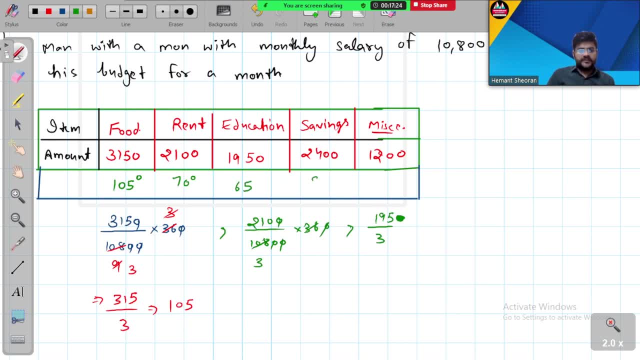 then the 240 over 3 will give us 80 degree. then 120 over 3 will give you what? a 40 degree, yes or no? yeah, is it clear? so this is what we call as a central angle. we calculated the central angle for us. 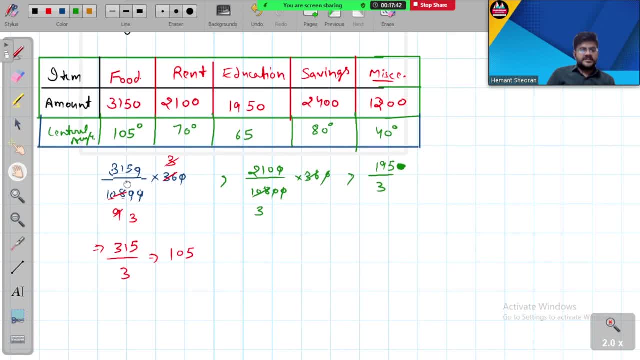 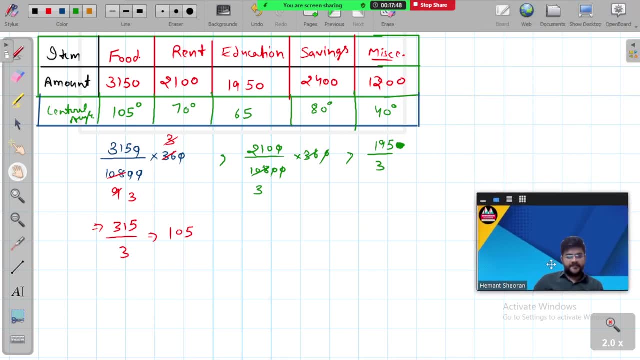 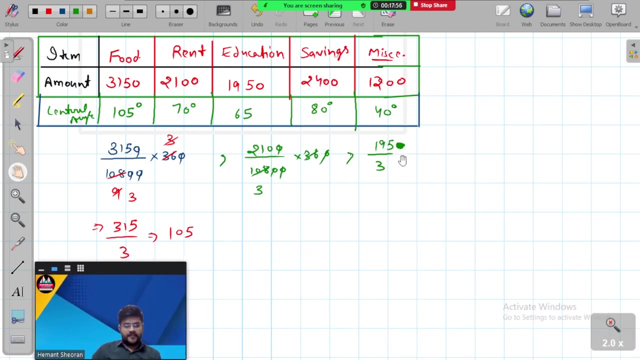 okay, now we can represent it in a circle, yes or no? yeah, okay, how are you going to do that? okay, so first we have to use a compass and then we are going to draw a circle first. yeah, let me check if they have a proper circle, so let me just draw a circle first. 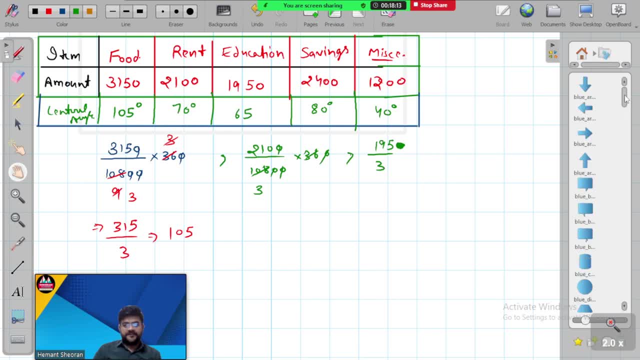 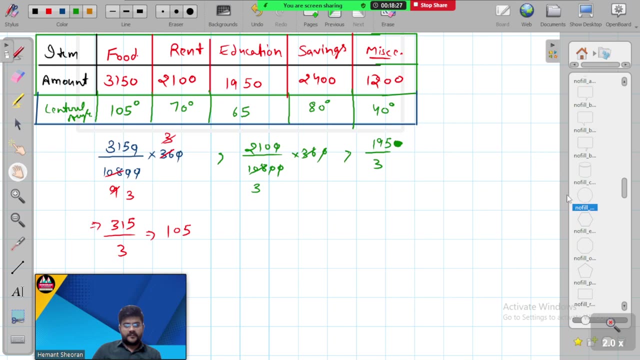 okay, so first we have to use a map 1 and then you just do like, let the your circle and next taking the metric right. and after doing that, what are you going to do? you gonna here, yes, keep the spread side distance. and then you want to make sure that you are done the surface, yeah, good. 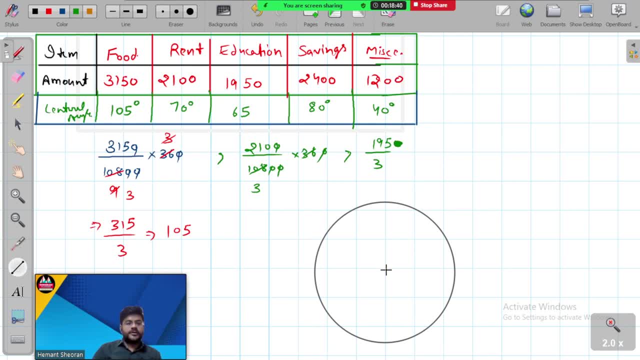 i want make it. lets say, put up horizontal, put the horizontal radius over there, get it. let's say, this is the center we got approximate, over here you will have your center, yes or no? then, yeah, this would be this horizontal radius for you, get it, and later on what you will do with this. so next, we gonna put, we gonna put. 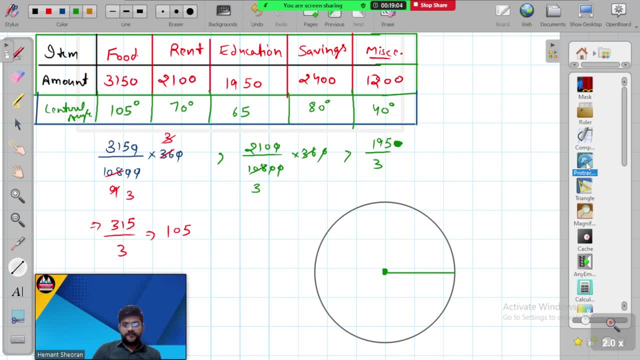 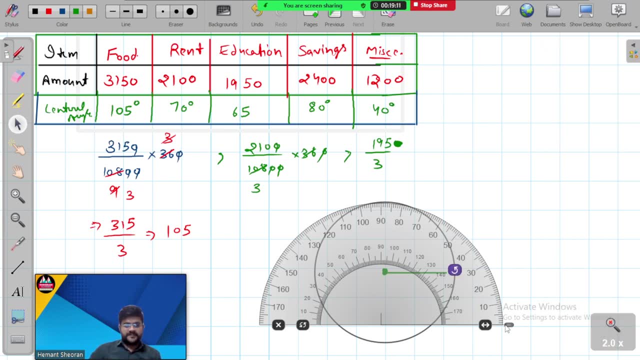 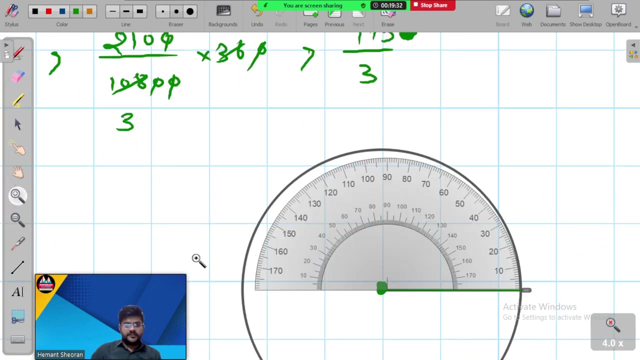 a compass now let, oh, not, not the compass protector, sorry, so we have this protector for us. is it possible to reduce the size? let me check. yeah, you can using the two arrows. okay, perfect, i think it is better let's zoom in a bit over there. okay, so we have it, and perfectly over here. 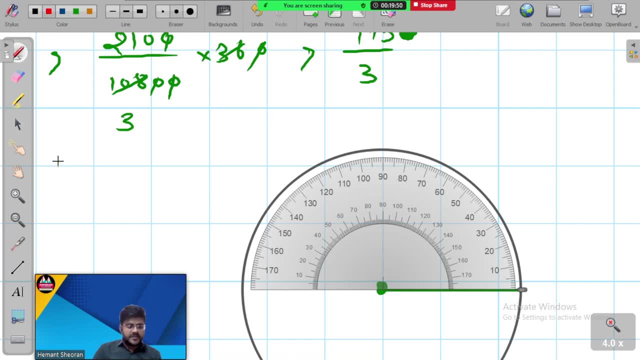 and then we use that line, then we use: so what angle? what angle? we have 105 first. so from where you will start the counting? we will start the counting from zero and this from here you will count. okay, so it is zero. then ten, twenty, thirty, forty, fifty, like one hundred and five, comes where a one hundred and five comes. 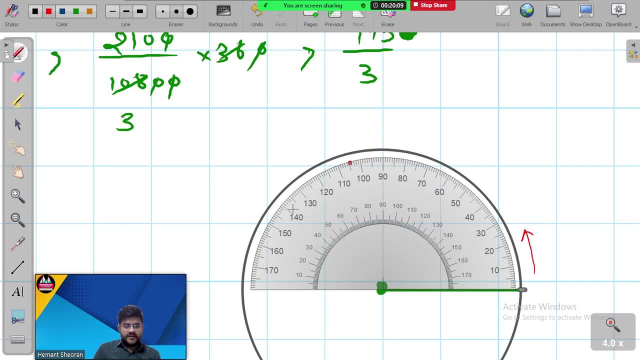 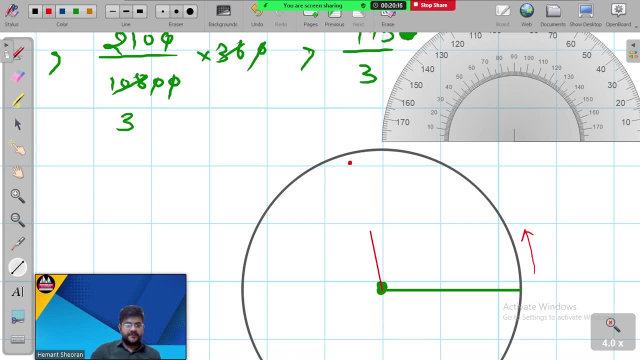 over here. yeah, then i will like put it aside and then I am gonna make a straight line for this: get it. Yeah, Okay, this way we go to 105. And yeah, we have 70.. this 105 is for what it is for food? okay, get it. then, the later on what part you will do. 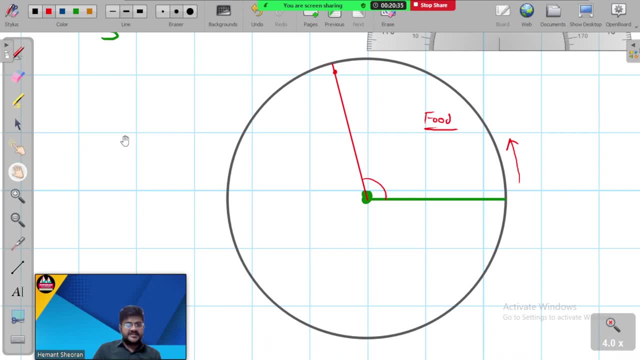 like, if we move to the next part, it is a 70 degree you have to create. so how are you going to create a 70 degree? now we use that second line and then put our protractor adjusted to there and then we measure. perfect. so this way we gonna do it. yeah, does it fits perfectly? I 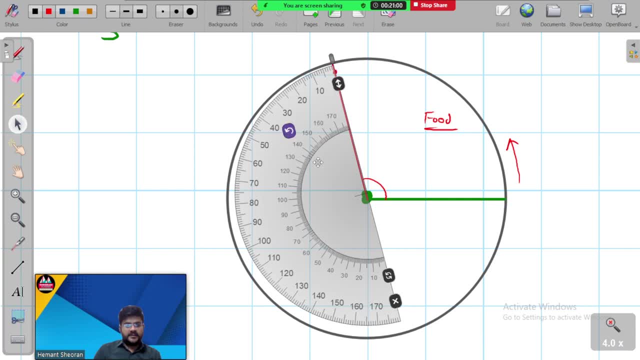 think now it's fit perfectly. yeah, a bit more, I need to shift. okay, it matches now. so what angle we have to create? we have to create a 70 degree angle now. so from again, like, this is like, you will start counting this way and this is the 70. 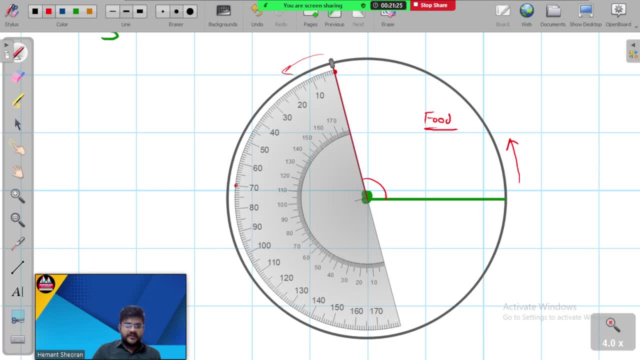 reading that you have. so over here you will get a 70 reading, yes or no? yeah, so again, you will shift it. let's- let's mark it from here, right here, it is 670 degree. get it. and the next reading, how, like what reading? you have to create a 65. let's make a 65 reading right now. so how we gonna make. 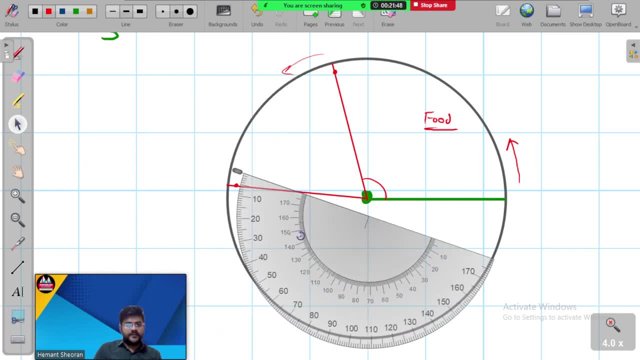 a 65 reading. let's go. what reading you have to create a 65 reading? yeah, so we're gonna rotate it more the same way. we're gonna do that. I think it matches now perfectly. then, like we gonna do what. we're gonna mark the. what number? we're gonna mark the 65, I think, the next reading. 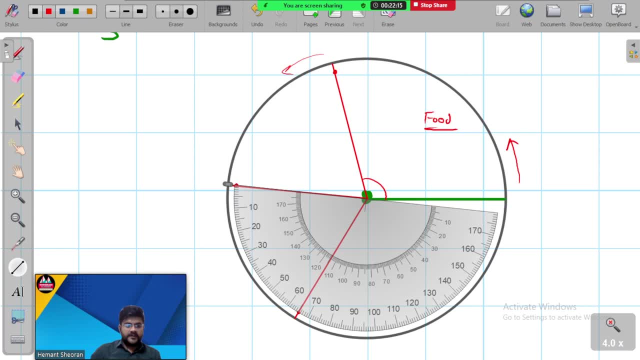 was 65. so it is over here somewhere, yes or no, and you're gonna make a straight line from there for it: yeah, it's 10.4 or something like that. so same way, we're gonna rotate it more. fifth: yeah, yeah, okay, then the next reading is for what? then the next reading is for 80. 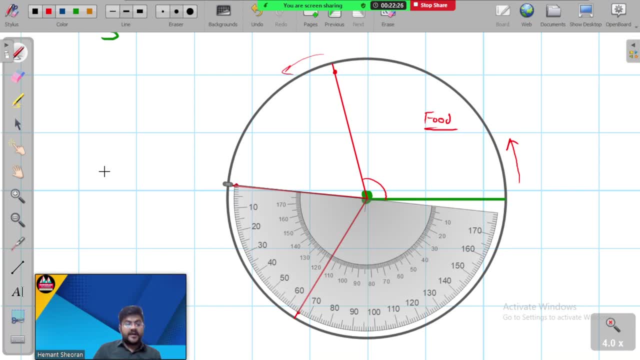 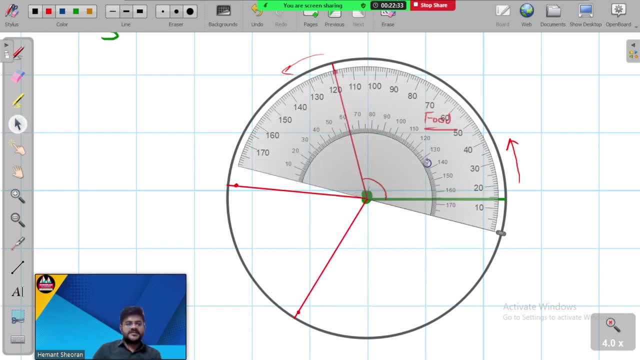 yes or no, yeah, and instead of doing this, if i tell you one more easier way, i like it just came to my mind, like, instead of making it again and again, like few, like just the two markings you can do easily. the first one was 105, next was, what next was was 70, so 175. you can mark it directly. 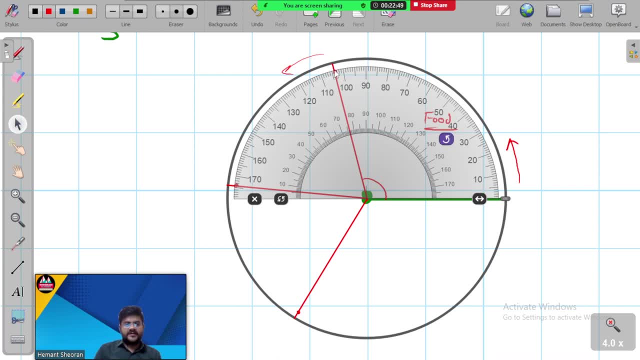 yes or no. the first point, you marked it as what? the first point, we marked this 105. next point, we will be marking as a hundred and uh, 75, yes or no? so that way also, like at a one time you can do two markings, get it, yeah. yeah. so that way also, like it will work. and from here only, 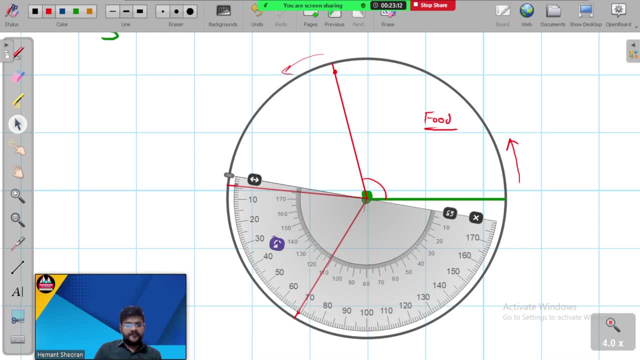 the sum of both angles is less than 180. it is it need to be less than 180? 180. 180 doors is less than 180. yeah, at a great height it gets less than 1850 different. okay, from here. we marked one of the angle. what was that angle? 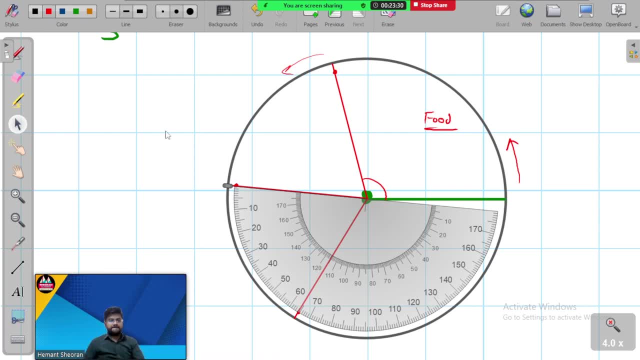 we just marked the 65- yes or no, and if you're gonna mark 80 as well, so what answer you're gonna have? for 80, yes um 145, 65 plus 80 will give us what 145, so 145 will be over here. yes or no. so we're gonna mark it directly, like that way also, like it will reduce your time, like you don't need to turn it, okay from here. we marked one of the angles. what was that angle? we just marked a 65 yes, oh, no. and if you're gonna mark 80 as well, so what answer you're gonna have for 80: yes, 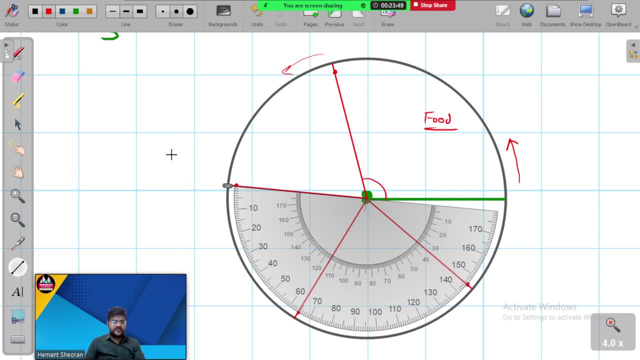 again and again. then the next thing will be: what? what angle you will have the 145 place for that one. we have to rotate it. yeah, is this correct? which one? the remaining part will be just a 40, my drawing, I think. yeah, it's perfect you. 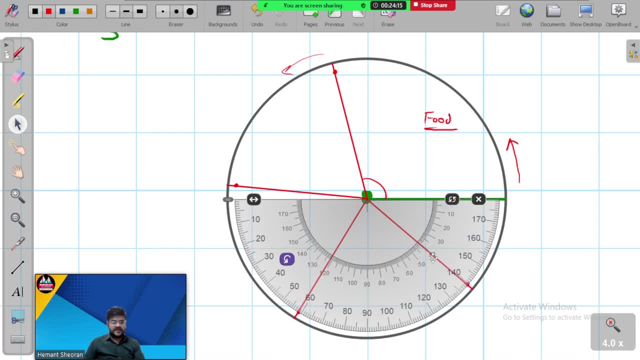 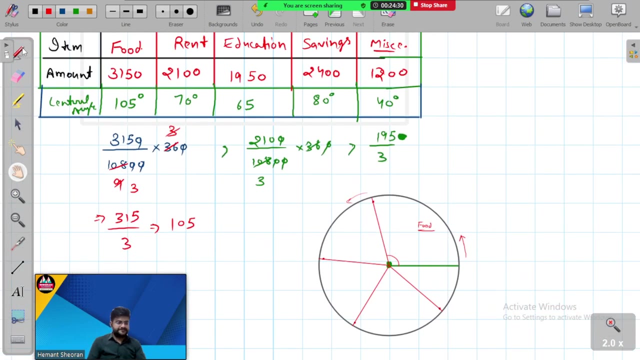 get the way. yeah, it is. it is perfectly fitting the 40. look at there. so now we can remove this from here and this is like the exact drawing that we were needing. and if I mark the places now perfectly, which thing was for what? so you can say this was for food and the next one was for rent and next one is 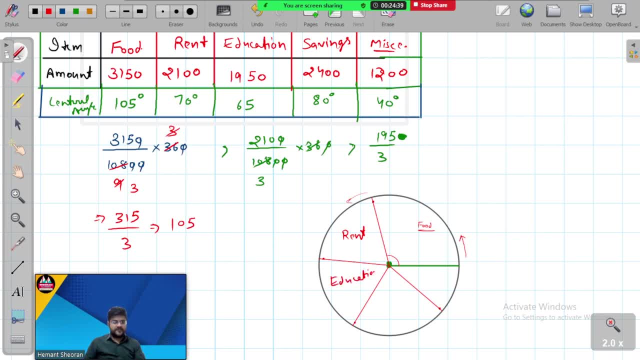 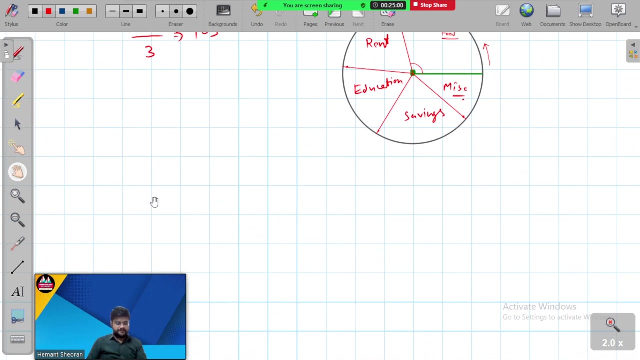 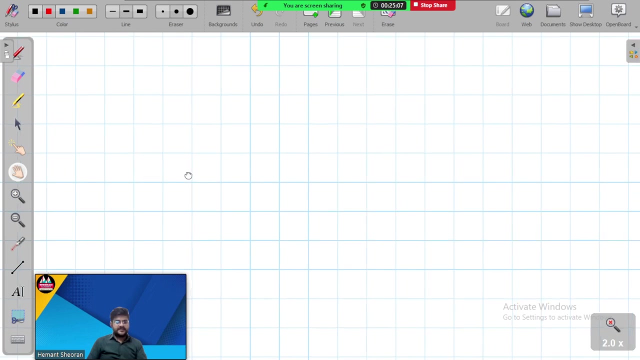 for education, yes or no? next one was for savings and next one was for miscellaneous. any confusion out there? no, no, perfect, okay, any confusion? no, so let's move to the next part. then in this one, can I try calculating the central angle? because, yeah, okay, that is. that is the part where 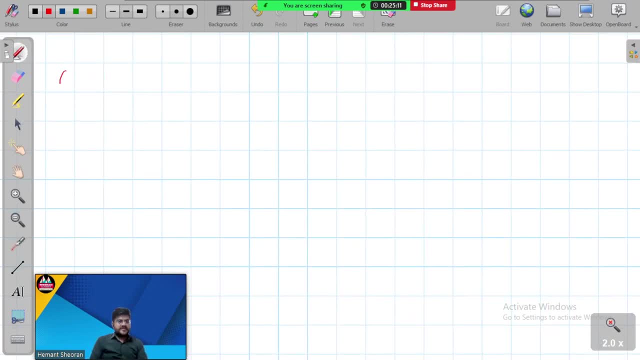 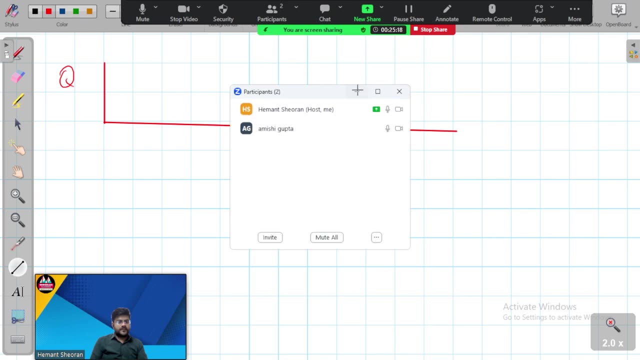 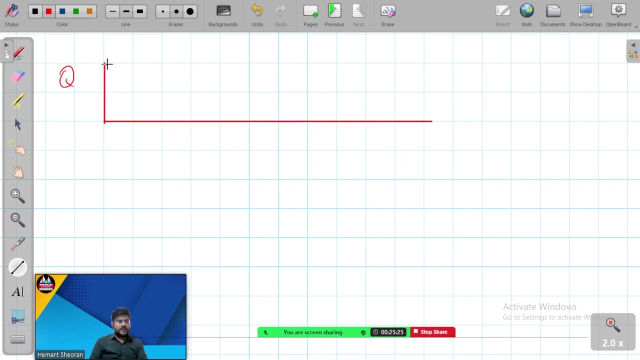 you have to practice, okay, okay, if I just give you a random dot, let's. let's make a table one more time, okay? so this is like the mode of transport. you can say: they have given us the mode and then the number of students who are choosing this mode of transport. 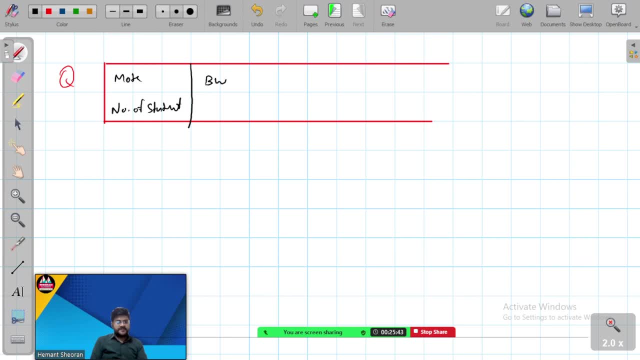 get it. so the first data is the number of students who are choosing this mode of transport. for a bus, so students were traveling by bus are 120. then students were traveling by the bicycle is 180. then the students were traveling by train: they are 240. and. 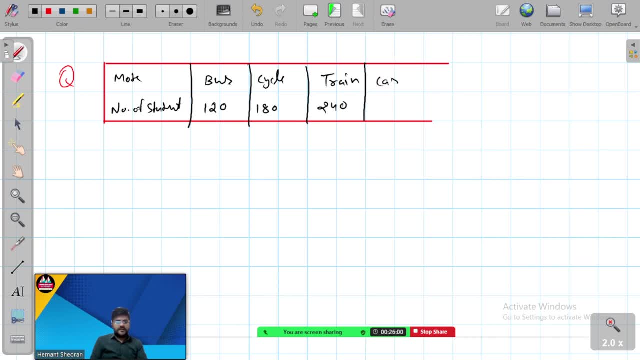 then the students were traveling by a car- they are 80. and then the students were traveling by a scooter, so they are 100. get it so if the total students are 720, so we have to do what we have to represent it in a pie chart. 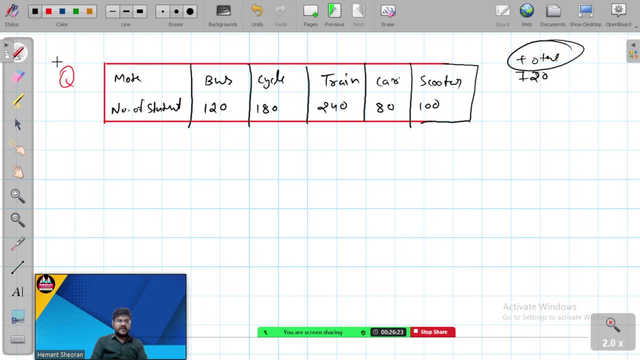 so just do the calculation of central angle. like the representation is a quiet time taking process. we can do it easily in exams. yeah, the total students are 720. so how are we going to find out the central angles so if we use that formula? so how are we going to find out the central angles so if we use that formula? set this in capital and take 20 times, which is 7. gladiators group. so this is the main depicts. set this жен et al counter by A and C candidates to choose Dealings each endHarmonically, except between C, as the C and D can be charged in expectation of C per. 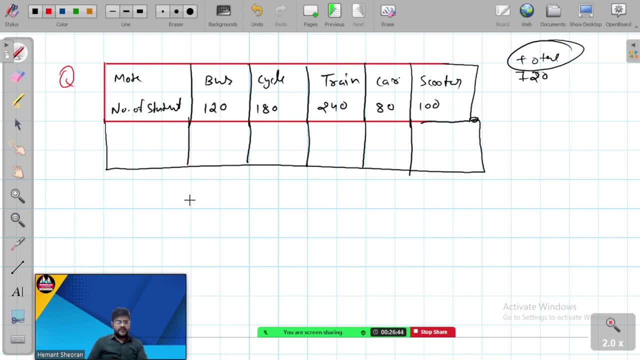 the formula says: what 120 over what 120 over the total, like just, we have to write down a fraction: fraction for what? fraction for the part we are taking divided by the total part that you have. so 120 over what? 120 over 720, you will. 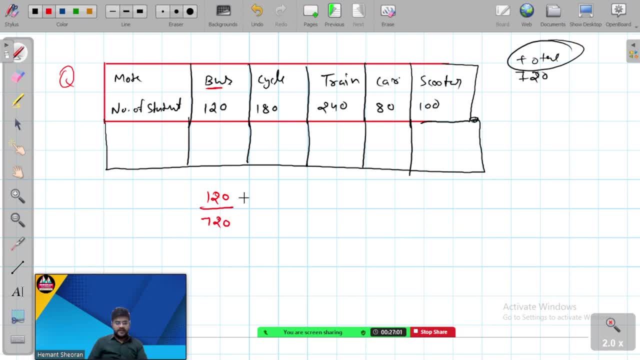 take yes or no and times it by what you gonna times it by 360, 1 over 6 times 360, so 60 degrees 360 will cut out the 72 at 2 perfectly, yes or no, every time it is going to happen. so we can say we get a ratio 360 and 720 will cut it out at. 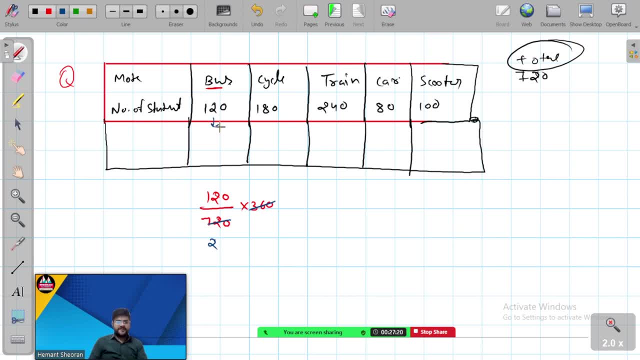 like a 1 over 2, so we just need to find out half of each. what will be the half of each? 60, 90, 120, 40 and 50. that's it like. that's an easier way. if you got up, if you got a perfect ratio, then you can do it easily. 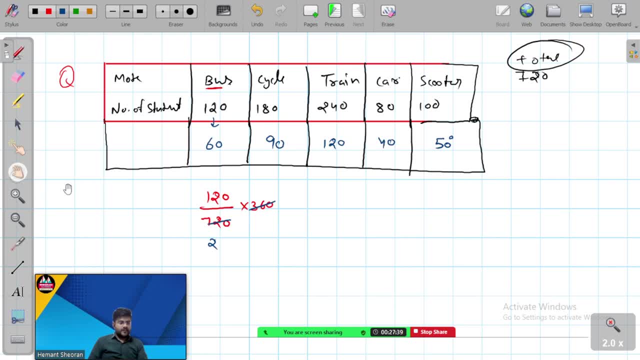 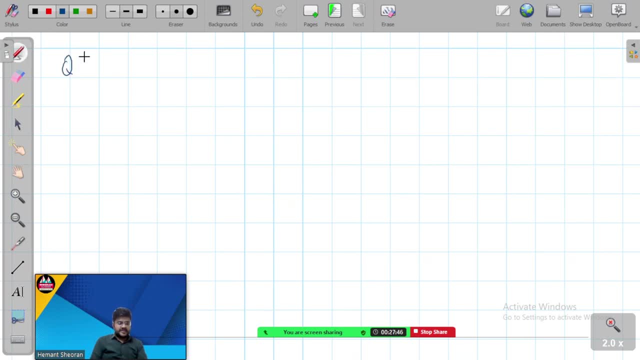 you, yes or no? okay, one more question where, like, the things will not work as smooth as they work for this one. the question says, like there are 216 workers that are working over there. okay, do I know this question or no? which one? this one? yeah, you have. you have to do it by yourself. there are 216 workers that work in a 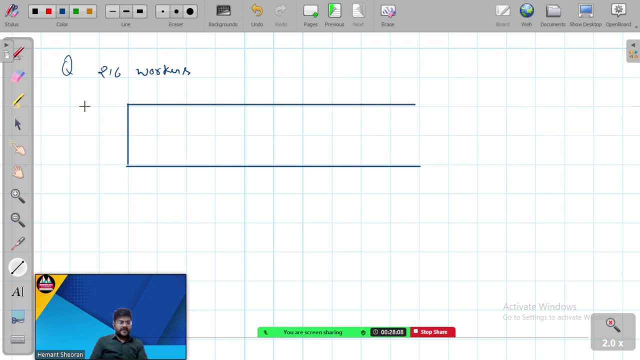 different cada. okay, we are dividing them in different cadders, you can see. so we will be writing the cada and down there you will be writing the number of workers in that cada. so if I start naming so few of them are labored a laborer, so let's. 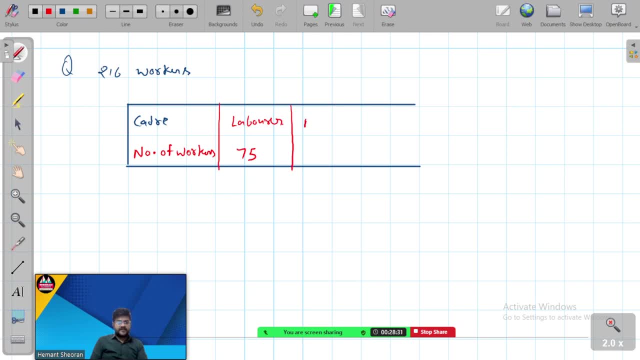 say 75 our laborer out of that, then some are mechanic, so let's say 60 our mechanic. and the next one is some are fitter, so there are 36 fitters. then comes the next data. the next one is the supervisors. how many supervisor we got? 27. then comes the 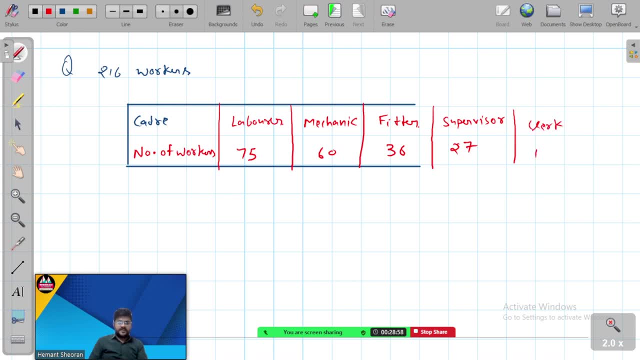 clerk? how many clerks? we have 18. just, you have to do the calculation. for it. be quick, calculate the central angle, and can I finish the tables? yeah, yeah, be quick. okay, sir, they can also include like percentage in the same topic. we will discuss few example on that one as well. so what? 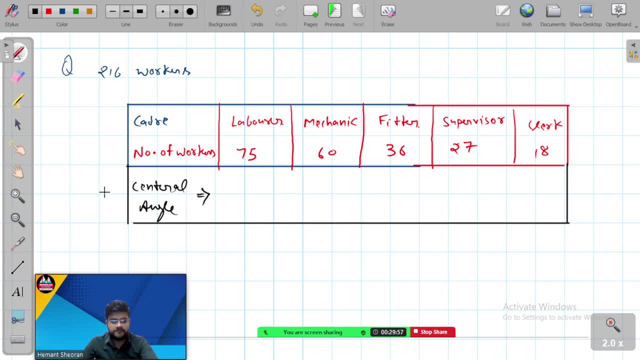 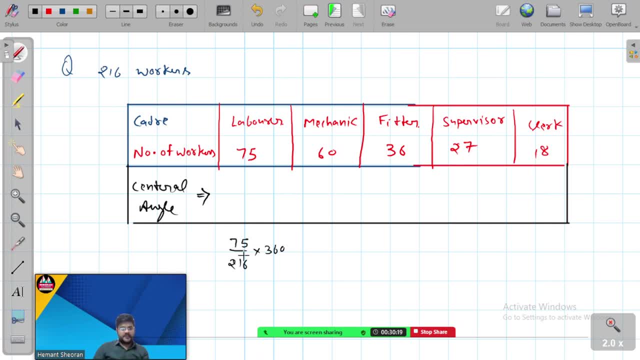 before, like moving ahead, what angle you got for it for this one, how much? i'm still sorry. okay, it'll be quick. 75 over 3 times 5. so 1, 2, 5. okay, you cut it out at what? so we can cut it out at. 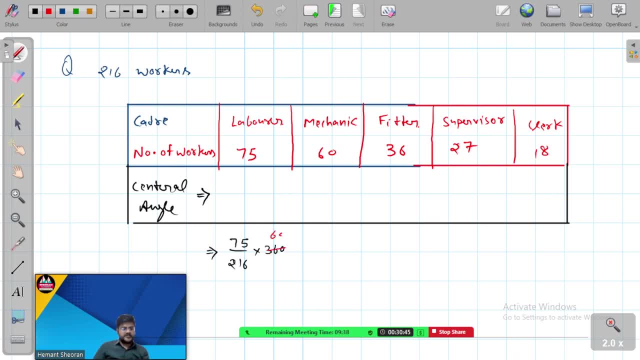 like 6 first, 6 times 60, and 6 will cut out at 36, yes or no. then 6 will cut out at 10, 6 will cut out at 6 again. then we can. we can cut it out at 6 again. then we can cut it out at 6 again, then we can cut it out at 6 again. 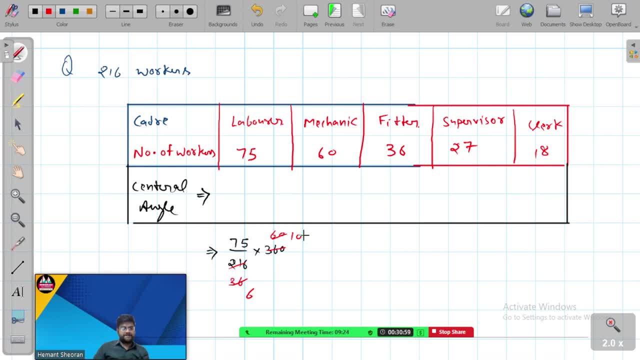 cut out like 75 with what with the? okay, let's cut out the 5 and 3, so we got a just yep, 5 over 3. every time you will be getting, so you can remember it. so for this one, like you can say, we just have. 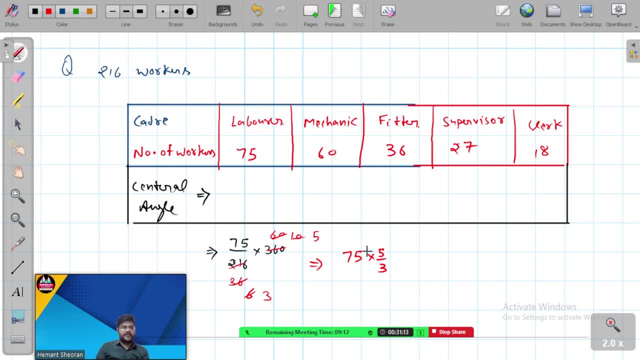 to do 75 times 5 over 3. every time you're going to multiply it each one by 5 over 3, because we just, if you look at there, we just focused on 360 and 216, so what you will get now, 75 will be. 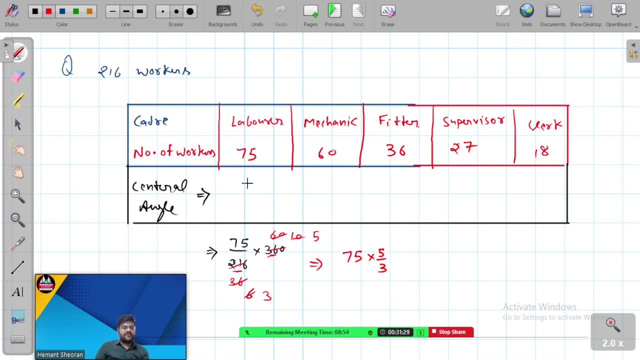 cut out by 3 at what 25? 25 times 5? yeah, perfect, 1 2 5. 1 2 5 is correct. go with the next one: 60 times 5 over 3. the next one will be 60 times 5 over 3 what you will get. 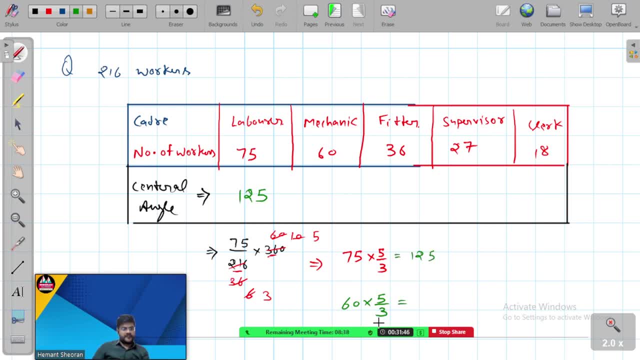 oh, um 100, perfect 100. the next one again by 5 over 3, 60, 60. next one: 5 over 3. um 3 will cut out 27 at 9, 9 times 5 is 45. same way 5 over 3, so 3 will cut out 18 and. 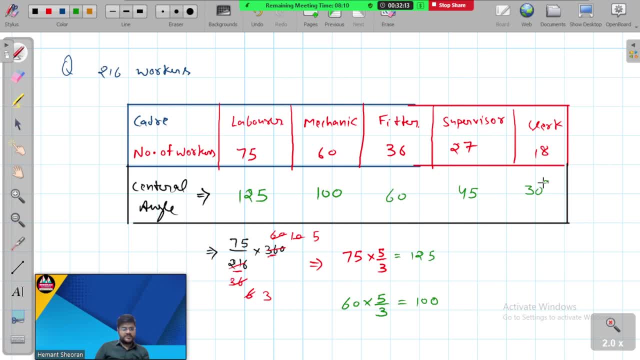 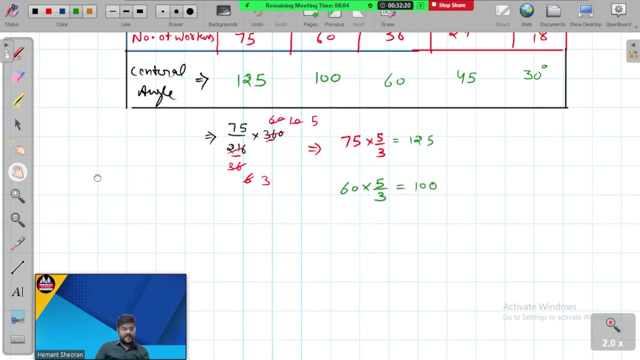 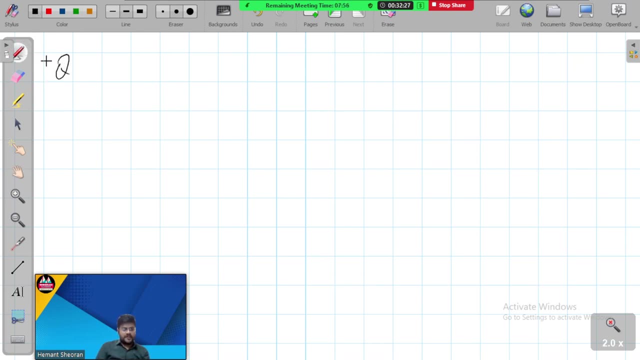 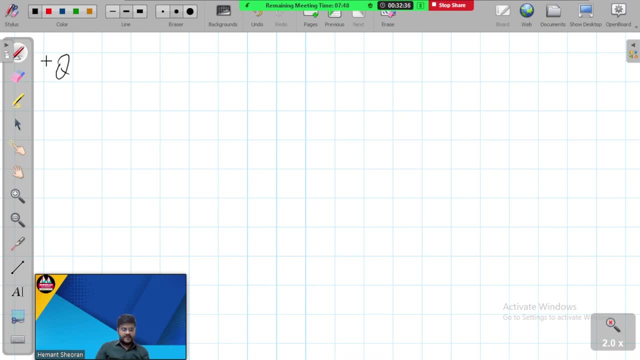 do it like after the class. let's work out like calculating the angle. okay, yeah, yeah, okay. so the next table that they are, uh, that is given to us, they are saying like the this table shows the expenditure in percentage. okay, on the construction of a house in a city. 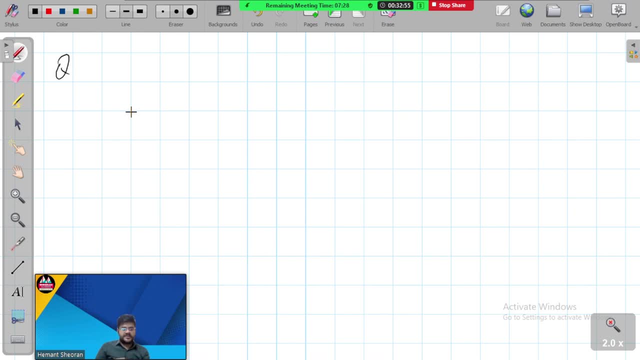 so how much? uh, they have like done the expenditure in percentages. okay, so we can say, like the first part that is given to us, what thing they per like made or what thing they purchased over there, and then expenditure, and then, if i make a table for it, so items that they purchase. first one is a brick. 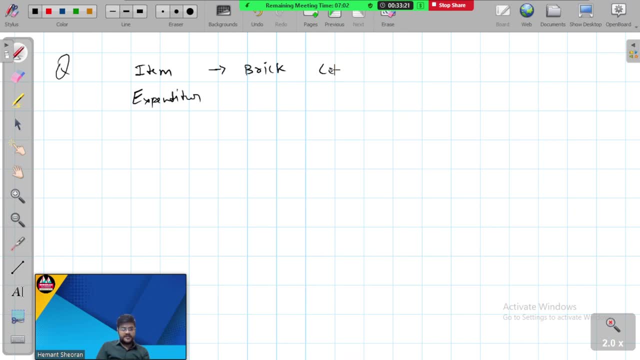 next one. they purchase the cement, then the steel, then the next one is the labor cost, and then comes, at the end, the miscellaneous one. okay, so how much they are, uh, spending on it? 15 percent on it, then for the cement, they've spent 20 percent. then for the steel, they spend 10 percent, then for the labor, they spend 25 percent. 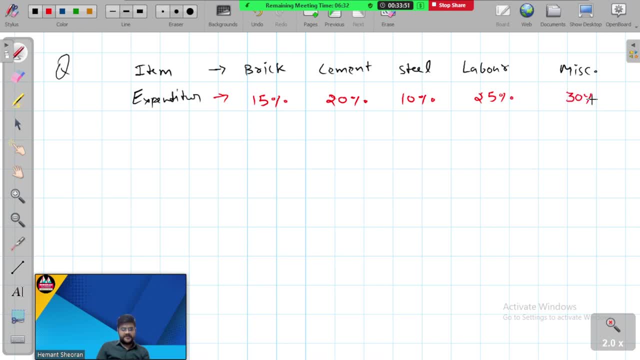 then for the miscellaneous they spend 30 percent. so we have to calculate the central angles. so i think we can easily do this. yeah, very easily, i think, because the denominator is fixed for it. what is that? hundred? hundred, because the percentage is always out of hundred. okay, 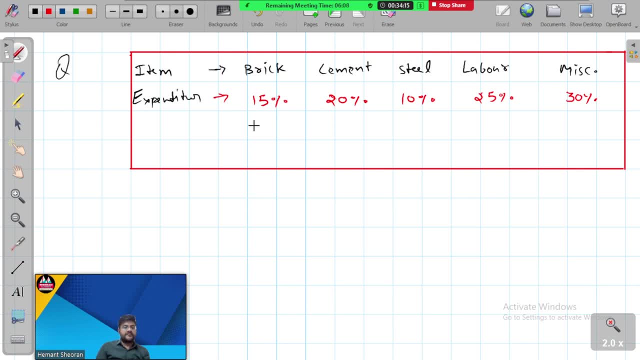 so we don't need a total data for it, or they will even not provide you because it will always be out of hundred. so how much it is out of hundred or what angle they will be creating this calculation so i can say for this one it would be 15 over what? 15 over 100 times by 360..